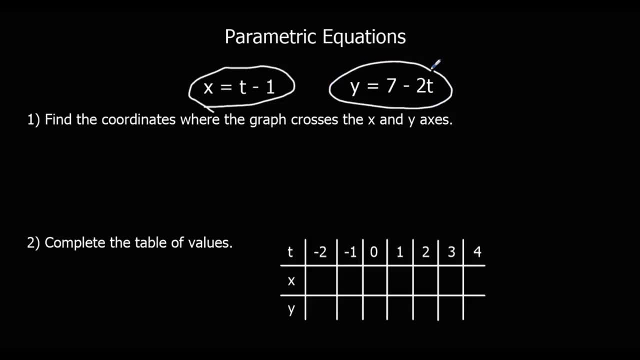 and an equation for y: y equals 7 minus 2t. So we've got two separate equations linked by t, the third variable. So the first question here says: find the coordinates where the graph crosses the x-axis and the y-axis. So we know it crosses x when y equals 0, and 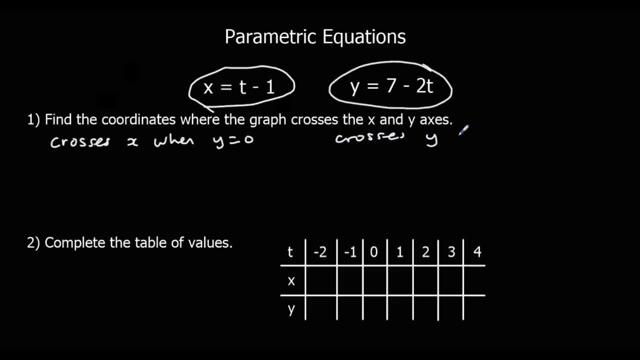 it crosses y When x equals 0. So to find out where it crosses x, we're going to substitute in: y equals 0. So we substitute that into the y equation. So 0 equals 7 minus 2t If we plus 2t to both. 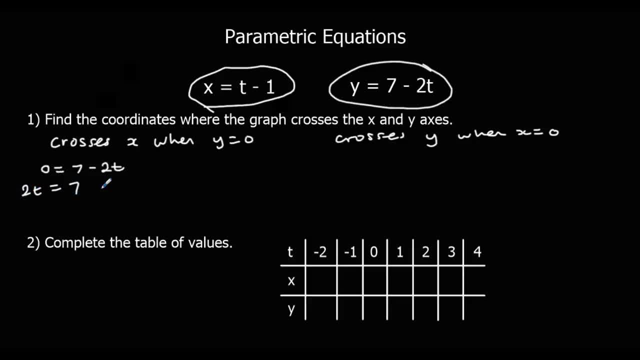 sides. we get 2t equals 7. And then divide both sides by 2. So t equals 7 over 2. Or 3.5.. So we know what t is, but we want to know what x is. So we substitute the t. 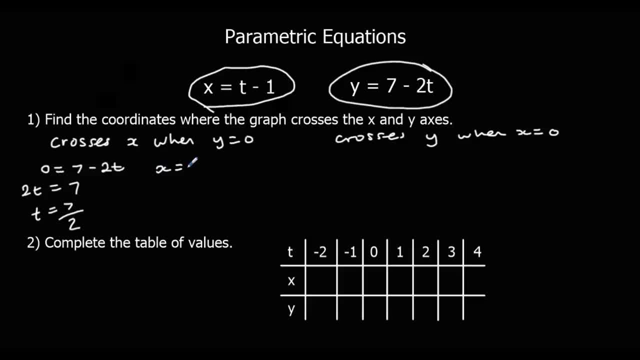 now into the x equation. So x equals 7 over 2 minus 1.. 7 over 2 minus 1 is 5 over 2, or 2.5.. So it crosses x when x is 5 over 2, and y is 0.. So they're the coordinates of where. 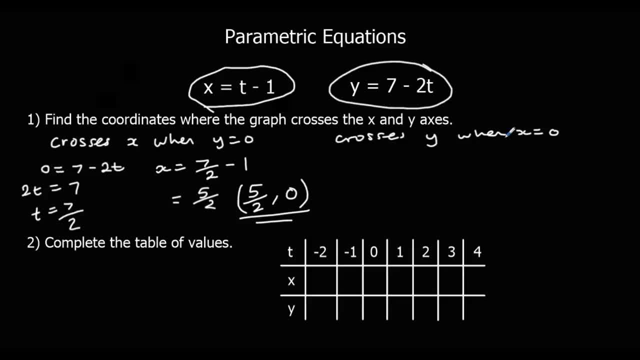 it crosses x. So if we substitute x equals 0 in, so we get 0 equals t minus 1.. So t is 1.. But we want the y, We want the y coordinate, So we substitute t equals 1 into our y equation: 7 minus 2. 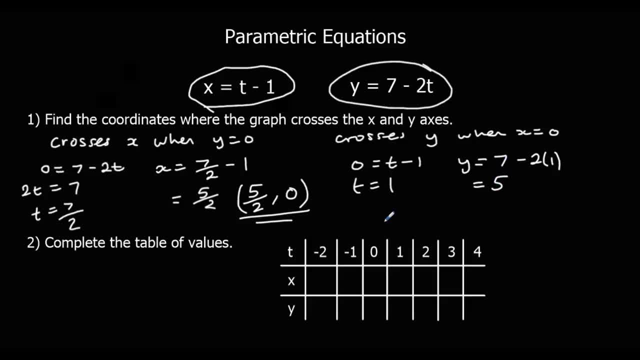 is 5.. So it crosses the y at 0 and 5.. If we need to draw a graph of a parametric equation, we complete a table of values with t at the top And then for each value of t we put it into both equations And then that. 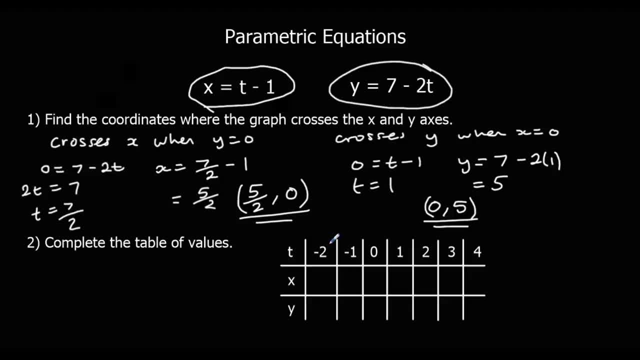 gives us the coordinates of each point. So if we substitute negative 2 in to the x equation, we get negative 2 minus 1, which is negative 3. And we put negative 2 into the y equation, So y equals 7 minus 2, negative 2s, So 7 plus 4.. So 11.. So when t is minus 2, we've got 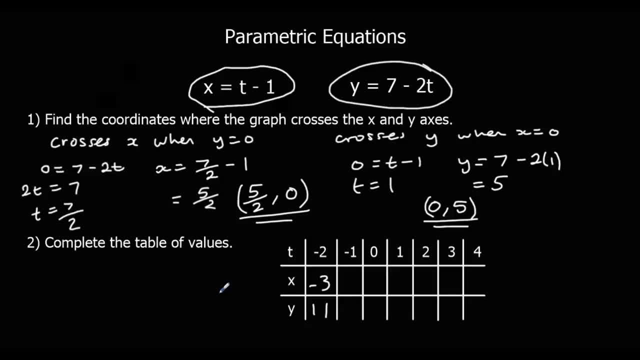 the coordinate of negative 3, 11.. And we can substitute all of these t values in, So if we put negative 1 in negative, 1 minus 1. And 7 minus 2 negative 1s, So 7 plus 2.. And 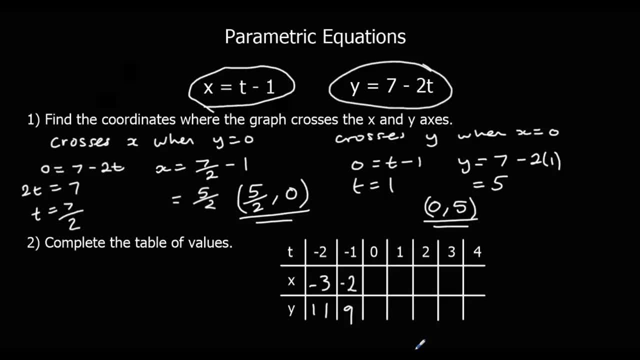 we can keep going, And then it will give us all our coordinates that we could plot on a graph, So 0 into both of them, 1, 2. And it's a straight line graph So we can see a pattern here. And then if 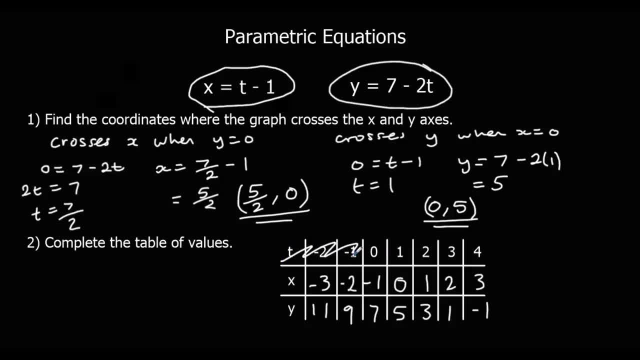 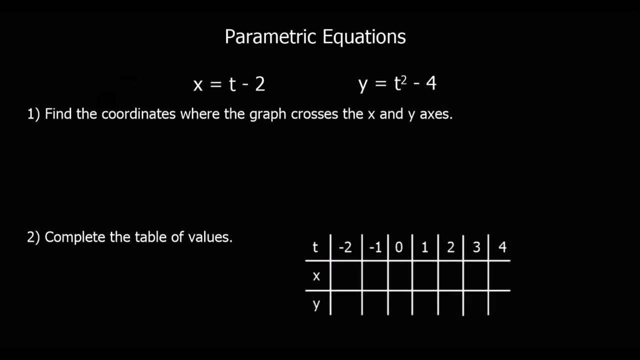 we wanted to plot the straight line graph. we ignore the t values and just plot our x and our y. OK, Here's another set of parametric equations. So find the coordinates where the graph crosses the x and y axes. Complete the table of values. So pause the video, give it a go and then. 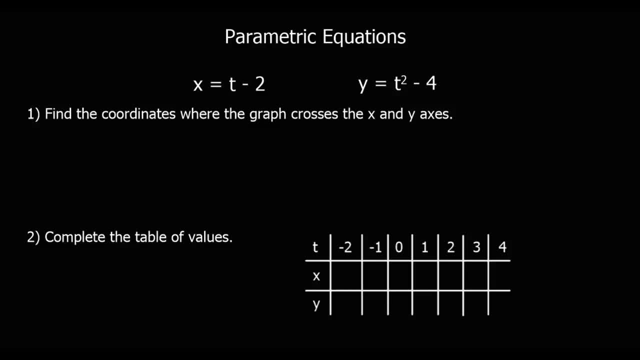 press play when you're ready to go through. OK, So it crosses x when y equals 0.. So when y equals 0. We've got t squared minus 4.. So 4 equals t squared. So t is square root 4, or the plus. 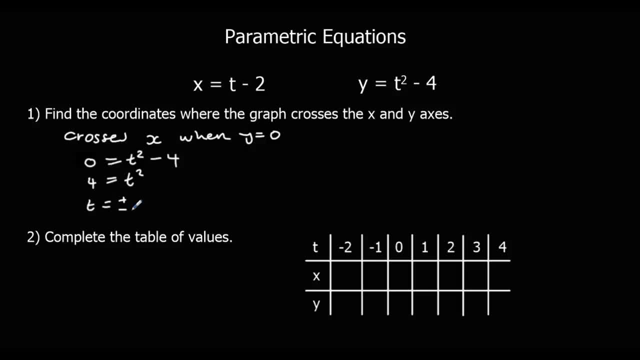 or minus square root 4.. So plus or minus 2 is our answer. So we've got two different t values. So we're going to put both of those into the x equation. So x can be 0.. 2 minus 2.. 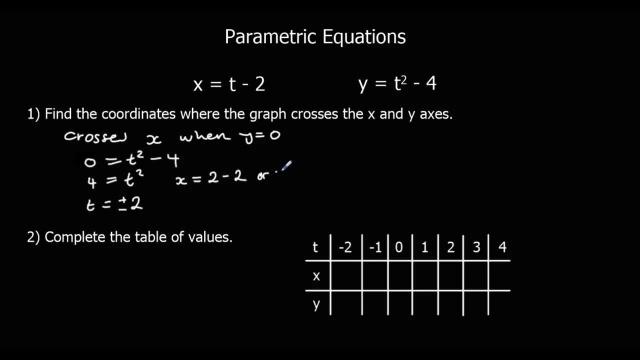 Or x equals negative 2 minus 2.. So x is 0 or negative 4.. So it crosses at 0, 0.. And negative 4, 0.. Find the coordinates where it crosses the y axes as well. So it crosses. 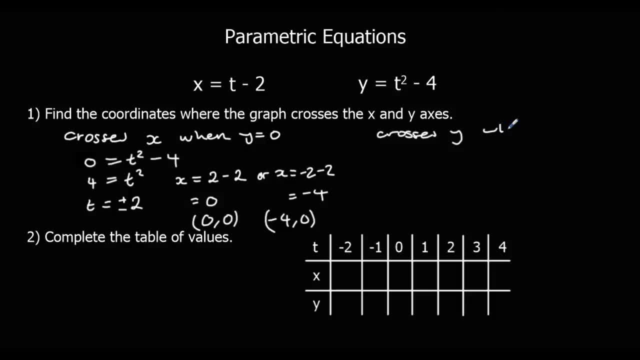 y When x equals 0.. 2 minus 2.. And x equals 0.. So when x is 0, we've got 0 equals t minus 2.. So t is 2.. And I think we already know this, because we've already worked this out. But y equals 2 squared minus 4, which is 0.. 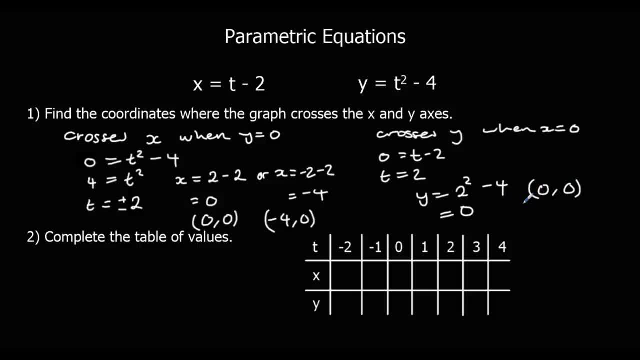 So it crosses y at 0, 0.. But we already knew that because we worked it out down there, OK. OK, Let's do this one tab at a time. OK, So if we take a negative 2 and a negative 2.. 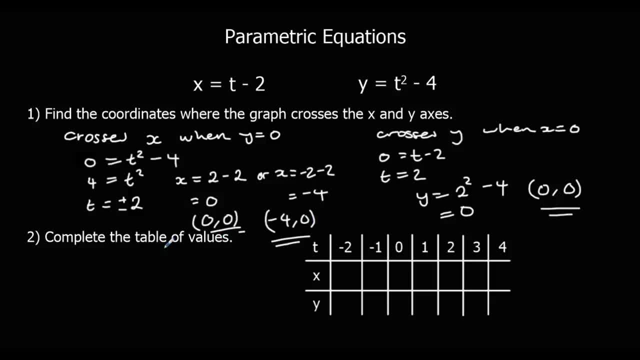 And complete the table of values. You can put in a negative 2, and take a negative 2.. Then let's do the remaining two And complete the table of values. So if we substitute minus 2, negative 2, into both equations, negative 2 minus 2 is negative. 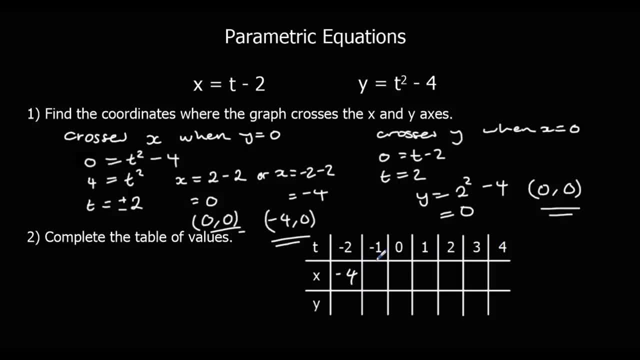 4.. If we just go along the x first, So negative, 1 minus 2.. 0 minus 2.. And we see a pattern: It's just a t minus 2.. 2 off the t, 2 off the t, t squared minus 4, so 2 squared is 4, minus 4 is 0.. 1 squared is 1, minus 4.